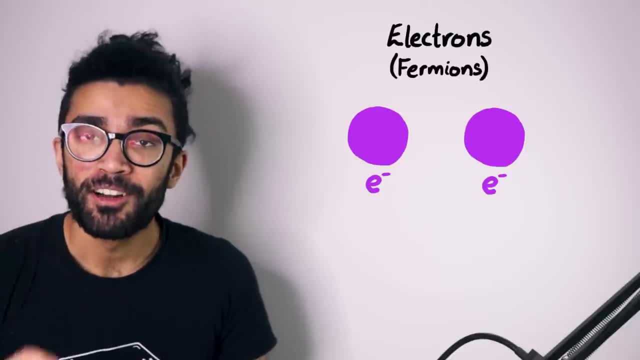 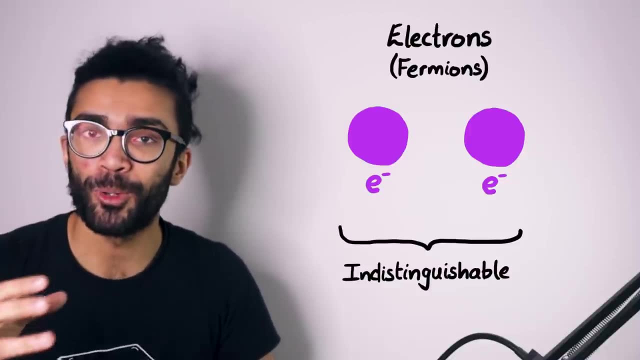 type of particle known as a fermion. Fermions are a type of indistinguishable particle, which means that two fermions of the same kind cannot be told apart from each other. they cannot be distinguished. they're identical because they have the same mass, same charge, same everything, but, moreover, 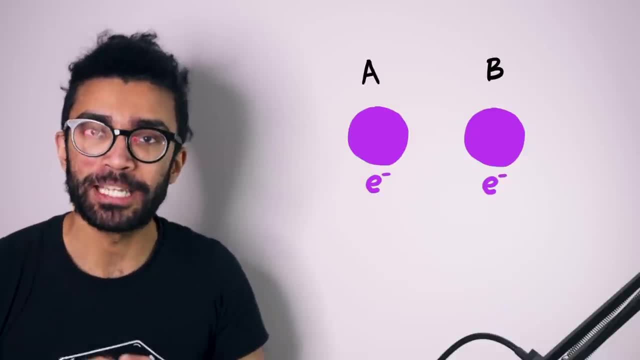 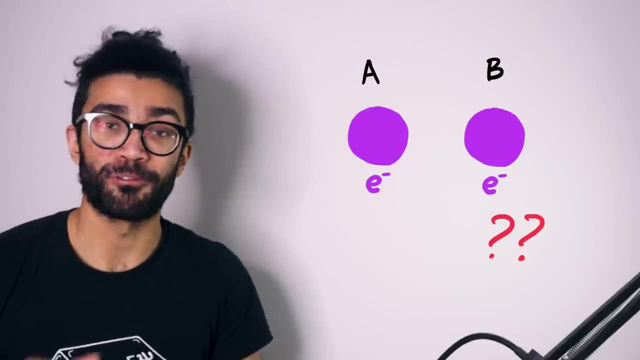 if we have a system of two indistinguishable particles and we leave it for a little while, then later on we have no way of knowing which particle is which. That's a slightly oversimplified description of a rather strange idea, so if you want to find out more about it, then please do. 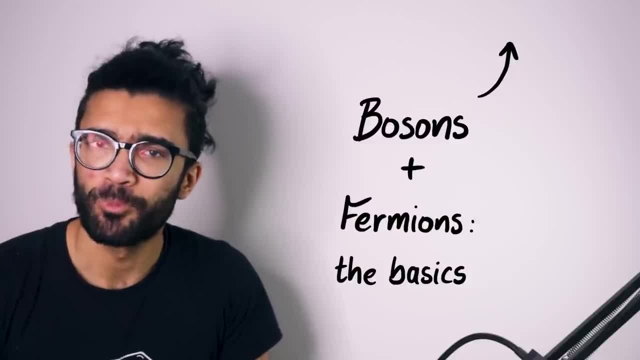 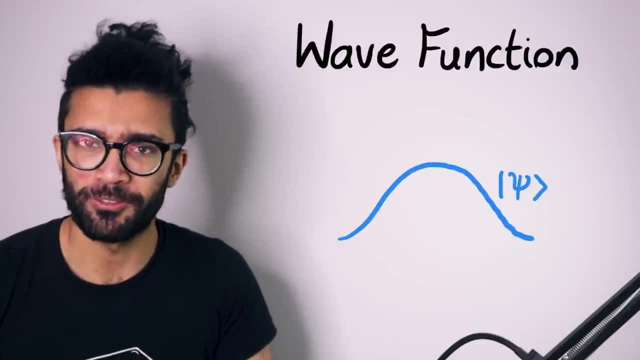 check out this video I made a little while ago Now. in quantum mechanics, with any system that we happen to be studying, we work with what's known as its wave function. This can be thought of as a mathematical function that contains all of the information we know about that system. 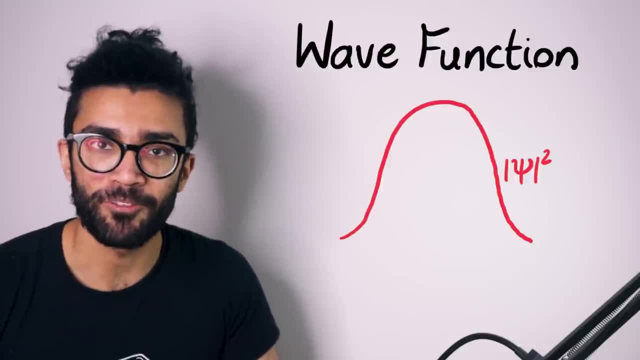 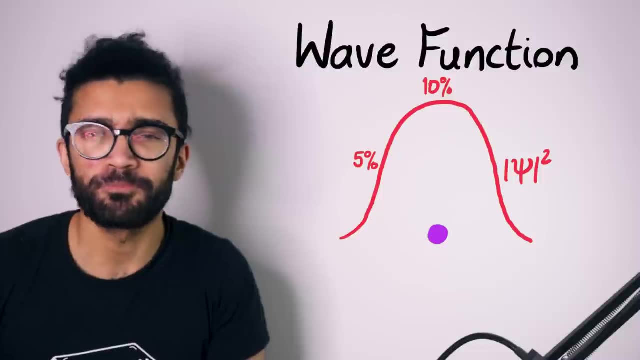 And when we take this wave function and we square it technically, we find its square modulus. then this gives us information like how likely we are to find the system in a particular location in space, for example, And for the two electron system we just mentioned a short while ago. 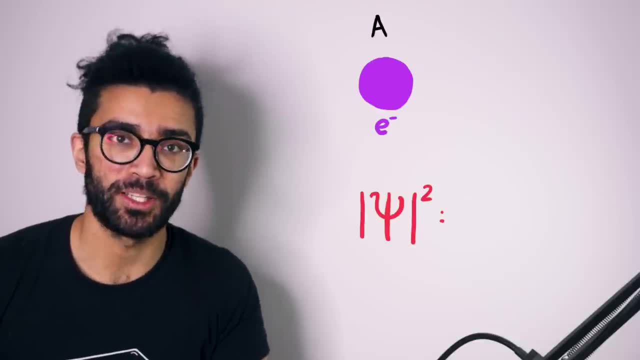 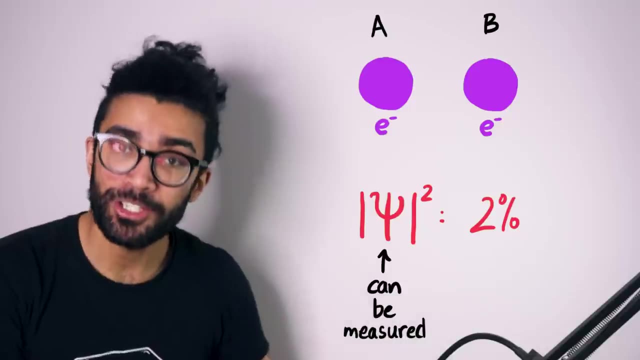 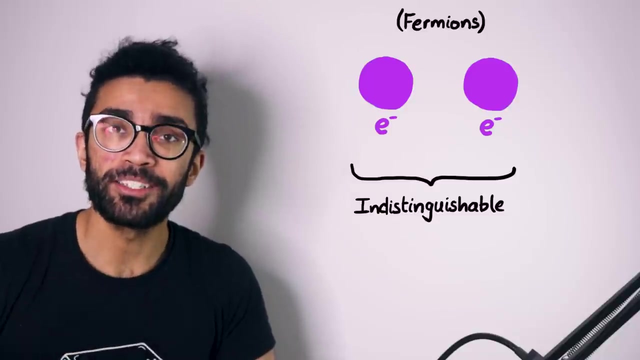 we could, for example, calculate the likelihood of finding one electron in this location and one electron in this location. The point is that the square of the wave function is something that we can directly measure in real life, And because these electrons are fermions, a particular kind of indistinguishable particle, we can encode their indistinguishability into the. 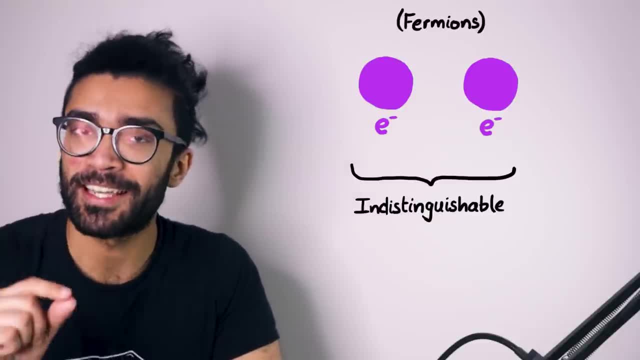 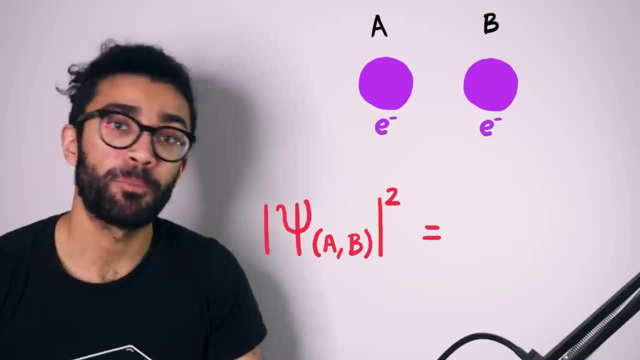 mathematics of quantum mechanics. The way that we do this is to say that the square of the square of the wave function is something that we can directly measure in real life. The system's wave function- again that's something that we can measure- must be identical whether our 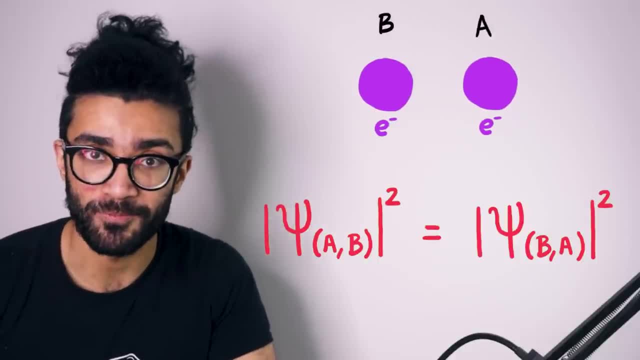 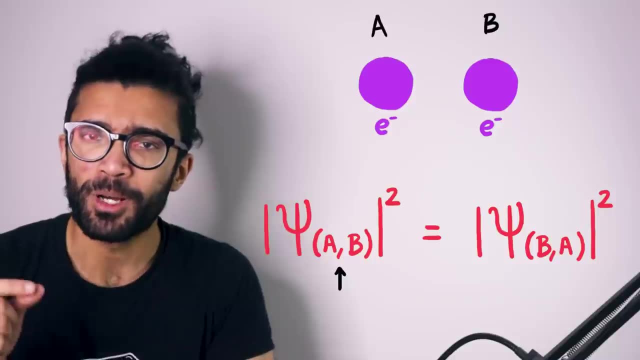 particles are in this orientation, or in this orientation, In other words, the square modulus of Psi. our wave function when the system is in orientation a- b must be exactly equal to the square modulus of the wave function when the system is in the orientation b- a. 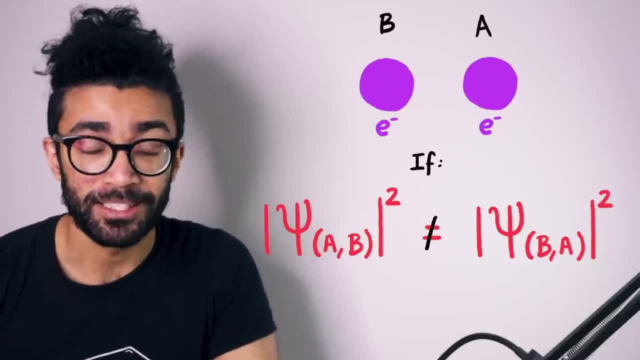 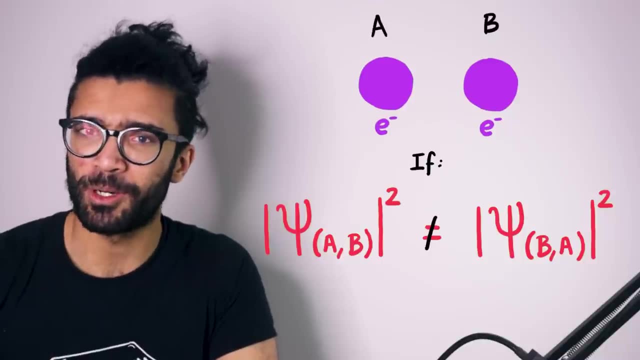 Because if these two quantities were different, if they were not equal, then there would be some way for us to measure it and therefore some way for us to tell which orientation the particles were in, therefore, meaning these particles were no longer indistinguishable. 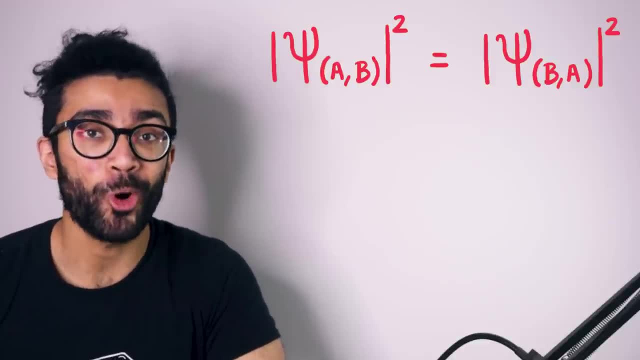 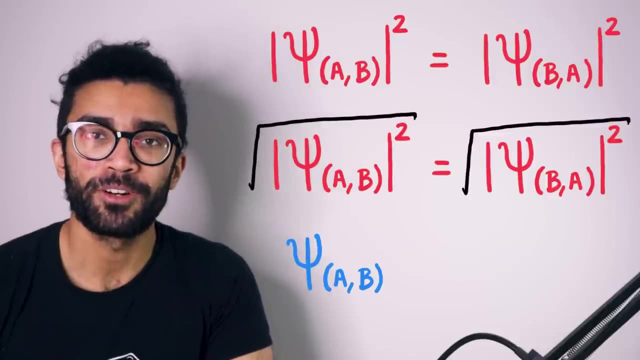 So this mathematical condition that we found here applies to all indistinguishable particles. Let's see what happens. when we take the square root of both sides of this equation, We find that the wave function for the orientation a, b must either be equal to the wave function for 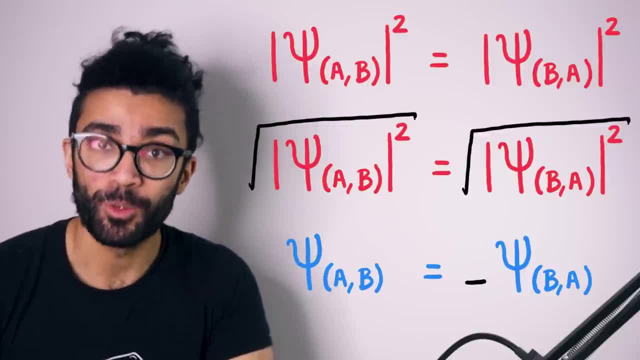 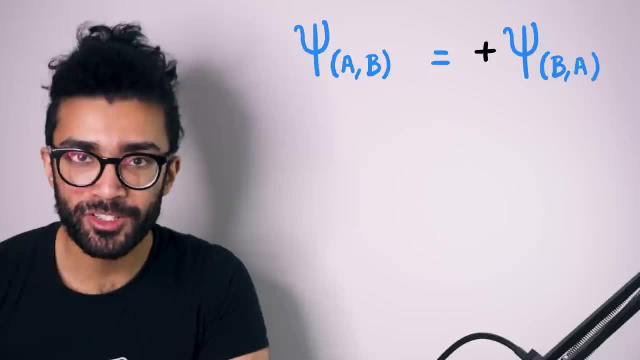 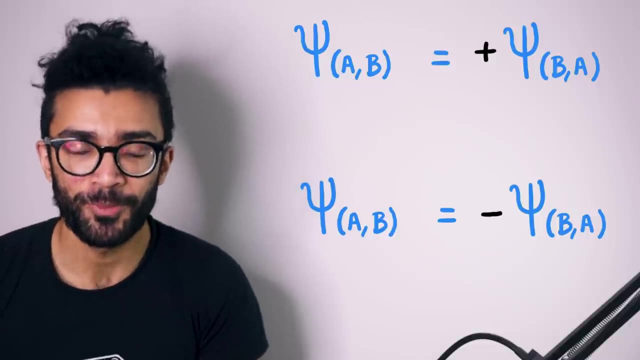 the orientation b a, or it must be equal to minus the wave function for the orientation b a. Another way to say this is that the wave function can be identical under particle exchange or it can become negative under particle exchange, and these conditions are referring to two different types of particle. 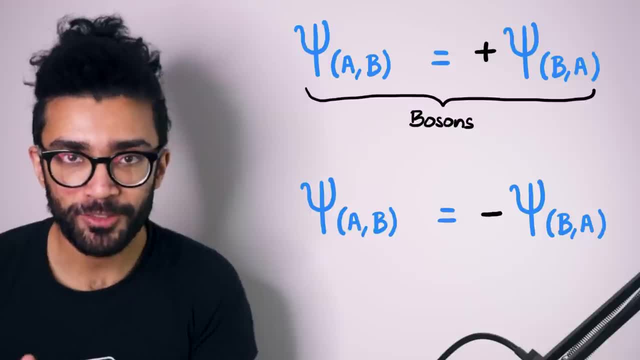 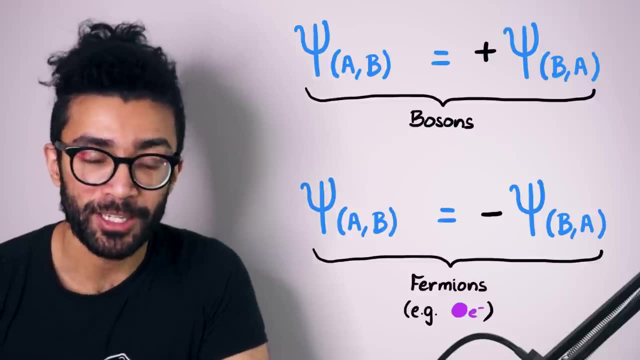 The first case is referring to a kind of particle known as a boson, and the second case is referring to a kind of particle known as a fermion. Again, we've already talked about electrons being fermions and we'll come back to them shortly. 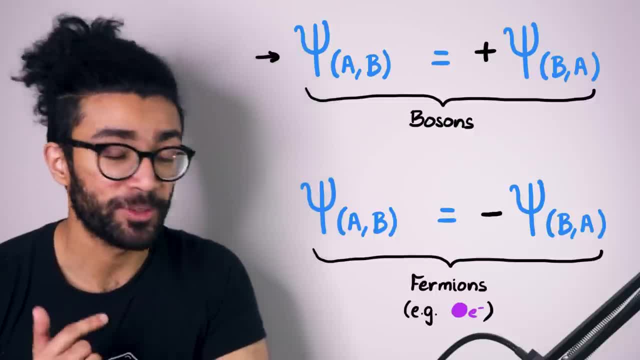 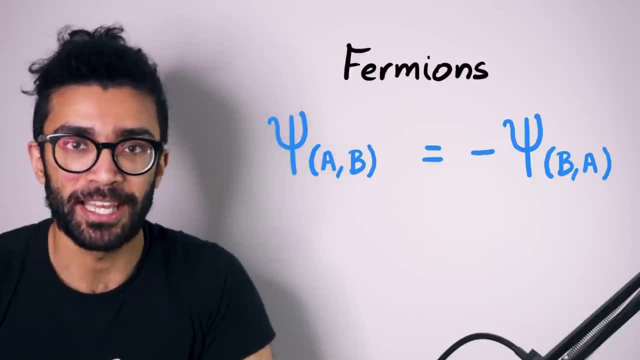 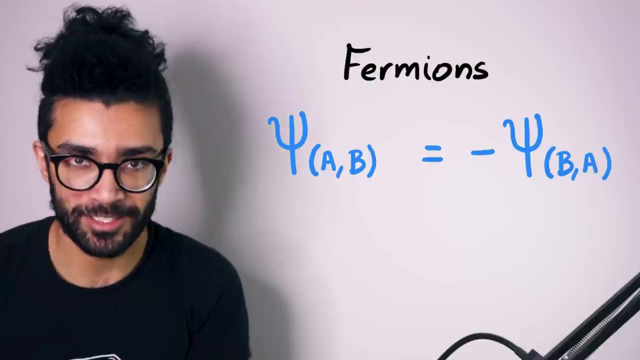 and I've also discussed bosons and their unique behaviors based on this mathematical condition in one of my previous videos on the Bose-Einstein condensate. So fermions, then, Our topic of today: Indistinguishable particles that have the property that their wave function becomes negative under particle exchange. 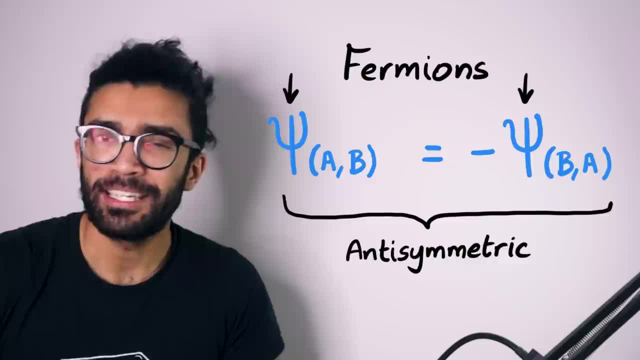 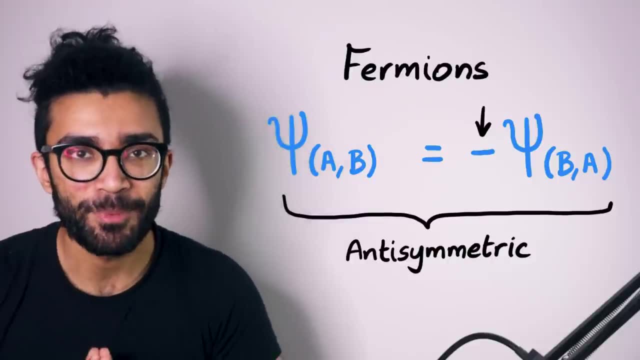 This is also known as an anti-symmetric wave function. It's essentially the same as before: there is some amount of symmetry, but it's anti-symmetric because it becomes negative. Okay, next let's imagine a very oversimplified system where our two electrons can be in two different energy levels. 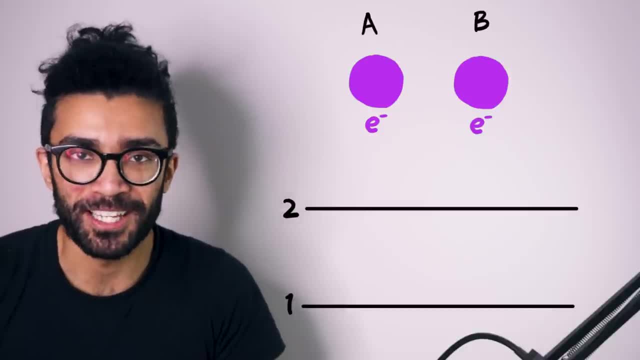 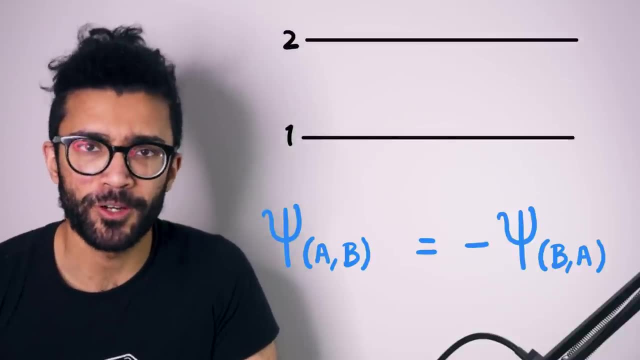 Let's call these energy levels 1 and 2. Pretty creative names. I know Now, following all the general rules of quantum mechanics, as well as this particular condition, that electrons, because they're fermions, should have an anti-symmetric wave function. 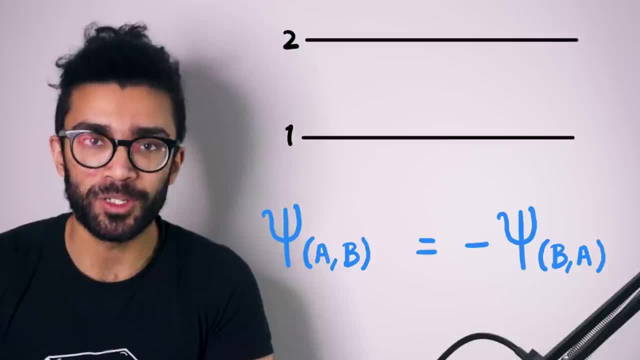 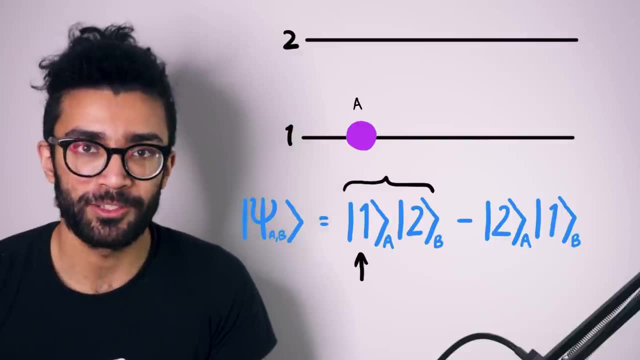 the only wave function that we can create for this system is one that looks like this: What we've got going on here is a superposition of two different states, One in which one electron is found in this energy level and the other is found in this energy level. 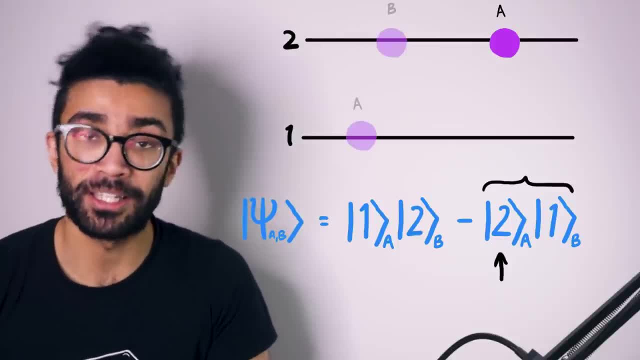 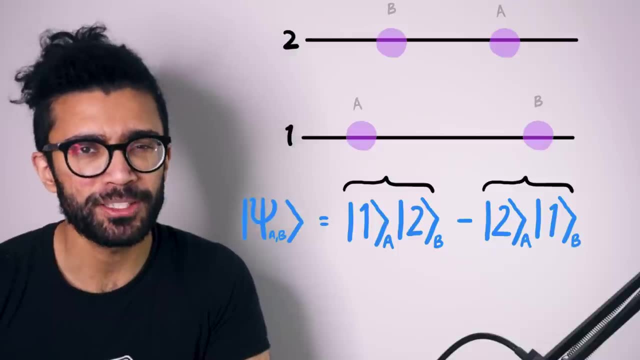 and the other state in which one electron is found in this energy level and the other electron is found in this energy level. Let's look at those. the negative sign that we see here is just a phase thing between these two superposed states and is not particularly important to us here. 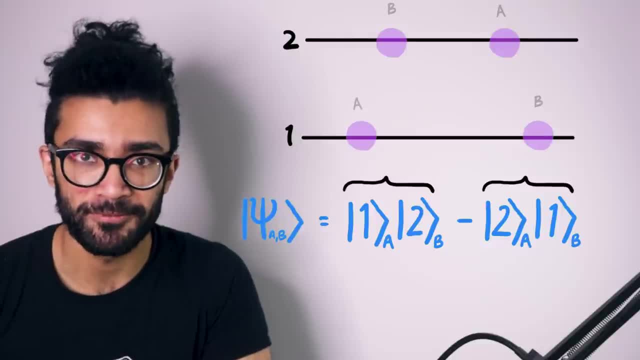 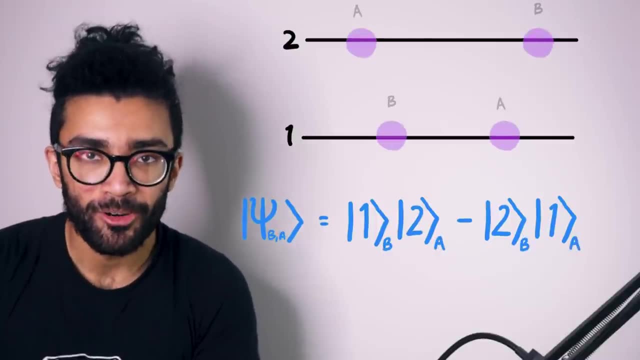 other than for the fact that this creates an anti-symmetric wave function, because if we take this wave function and we now exchange the two particles- a becomes b and b becomes a- then the wave function now is exactly negative of what it was before, which is exactly what we want we. 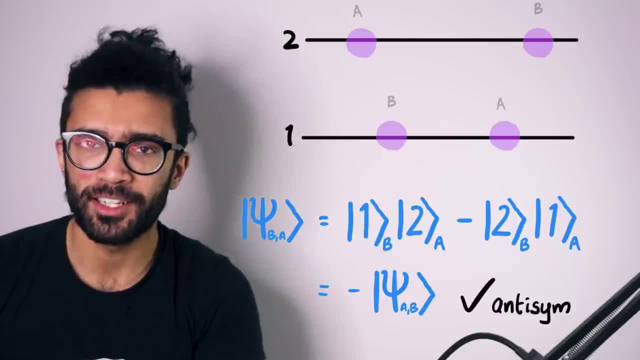 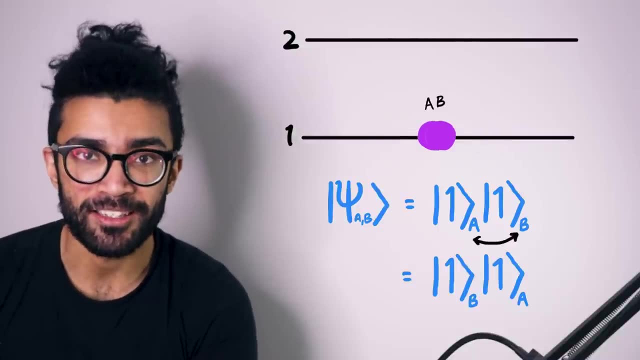 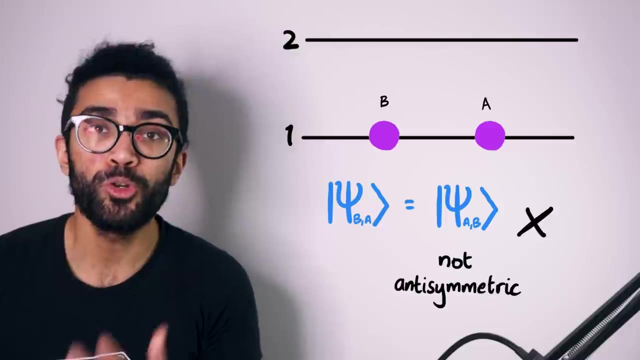 want an anti-symmetric wave function, whereas in any other scenario, for example if we were to find both particles in the same energy level, that wave function would look like this: under particle exchange it stays the same. therefore, it's not a fermionic wave function. it's actually a good bosonic wave function and it could be used to. 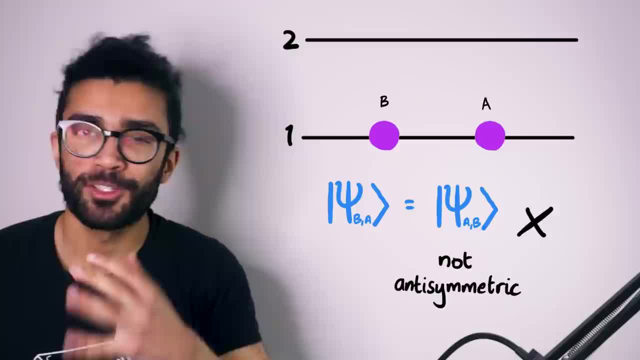 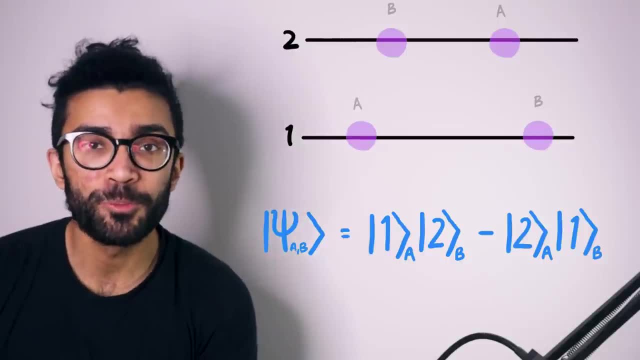 describe two bosons in a similar energy level system. so let's go back to our fermionic wave function, the one that is allowed for two electrons in this kind of system, because we've got a quantum superposition going on. and, by the way, check out my quantum. 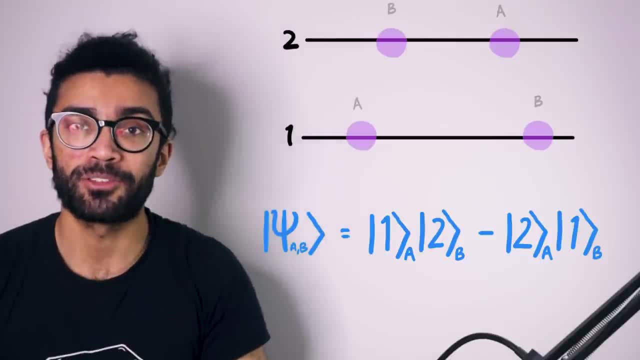 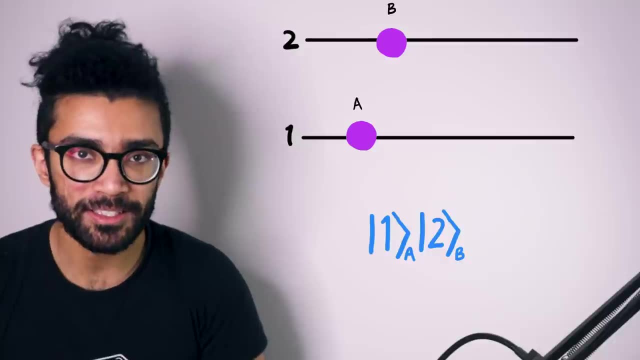 mechanics playlist. if you're unfamiliar with superposition, the fact of the matter is that when we make a measurement on this system, we will either find one electron in this energy level and the other in this energy level, or we'll find this arrangement. we will not find both electrons in the same. 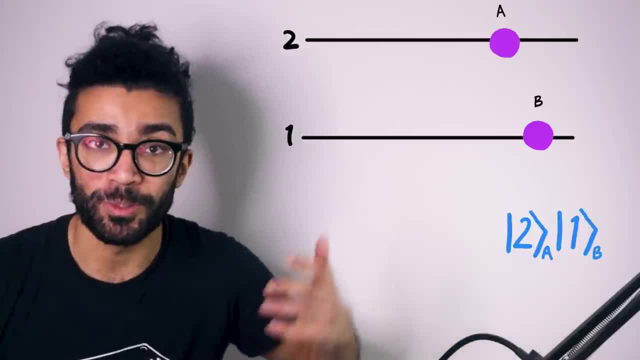 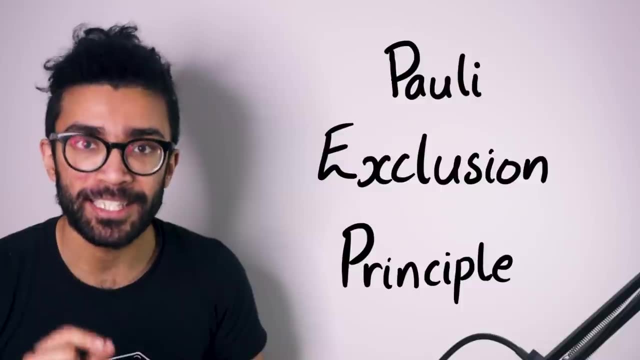 energy level, they can't be there. they could if they were bosons, but they can't be there because they're fermions and therefore what we've just seen is a very simplified way of visualizing Pauli's exclusion principle. this is a principle that says: 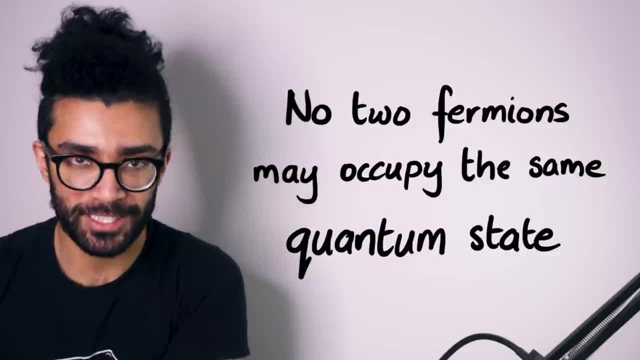 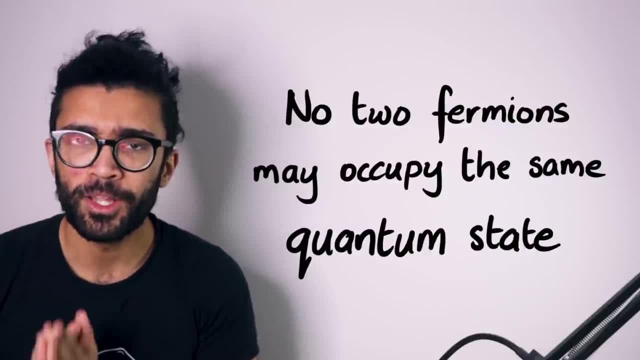 no two fermions can occupy the same quantum state. now, using our simplified system, we might be forgiven for thinking that Pauli's exclusion principle is telling us that no two fermions can occupy the same energy level. but that's not quite the same thing, and the reason is because we've got an 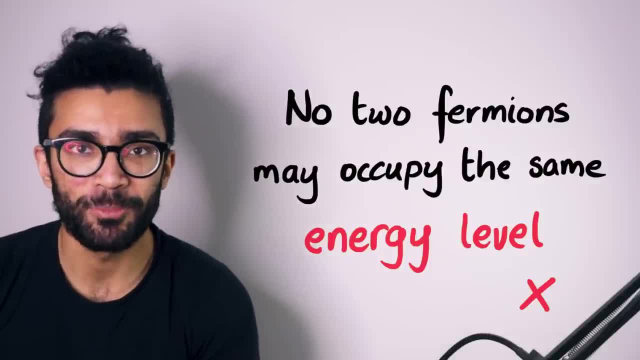 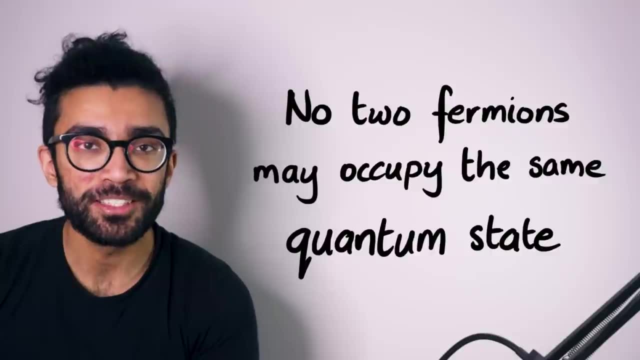 oversimplified system. if we account for the other complexities of quantum mechanics, then we find that no two fermions can occupy the same quantum state. so let's talk about what we mean by that. let's now consider electrons in atomic shells. so we've got a nucleus. 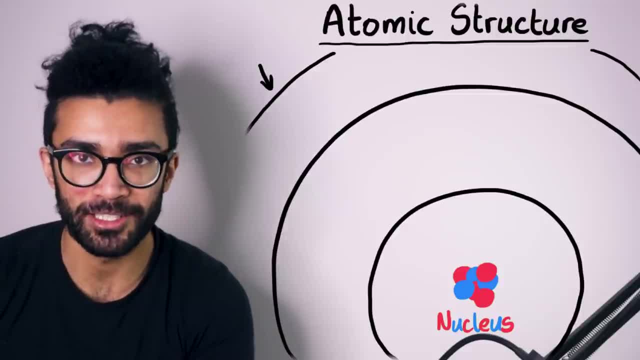 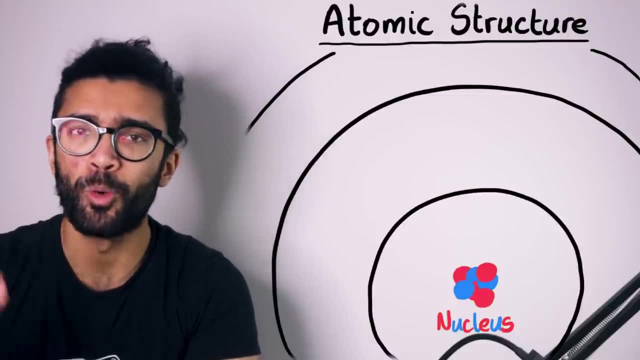 and we've got energy levels that the electrons can occupy surrounding that nucleus. if we were to believe what our oversimplified model from earlier told us, then we would think that the electrons could only be arranged- one electron per shell- and this is what atomic structure would look like. 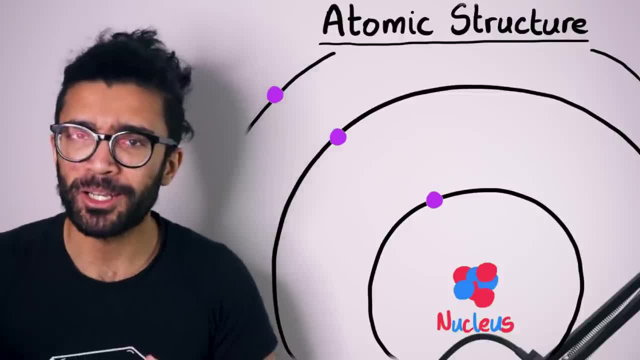 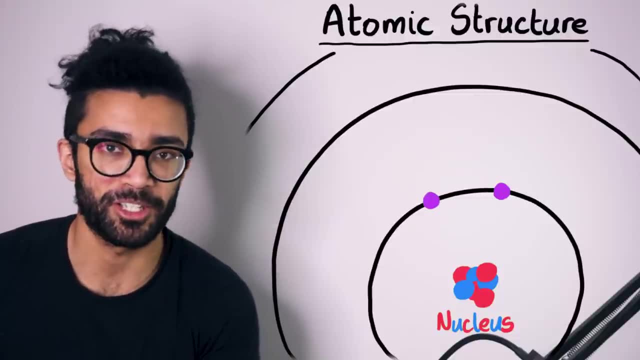 and that's not quite right, but there is some truth to it. it's not like all of the electrons are falling into the lowest energy level, however. in reality, the first shell can hold up to two electrons and the second shell can hold up to eight electrons, and so on and so forth. 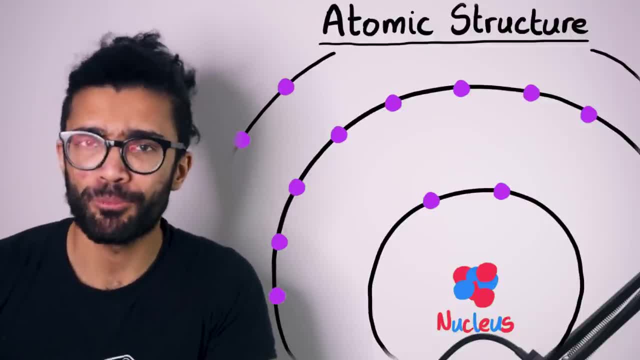 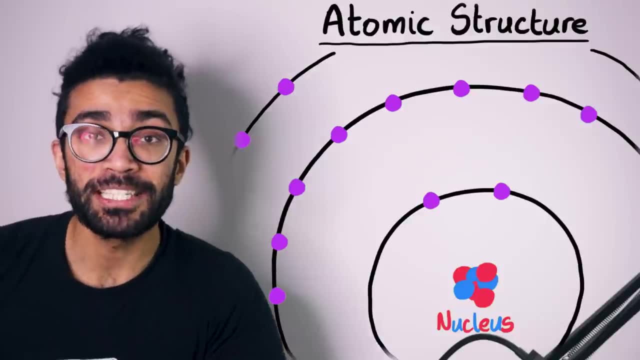 the reason is that electrons in each one of these shells have a few different properties and it turns out that, conveniently, we can represent each one of these properties with a simple single number. we've actually seen one of these numbers already. it's known as the principal quantum number and it represents which shell the 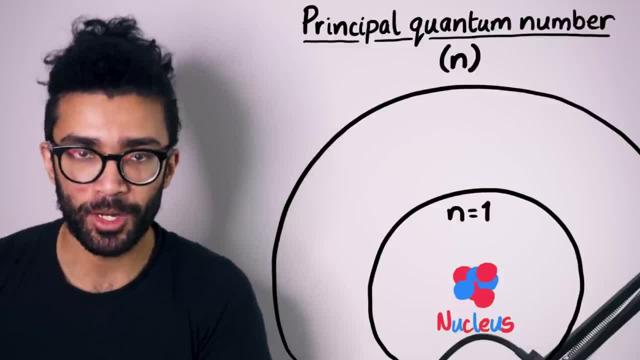 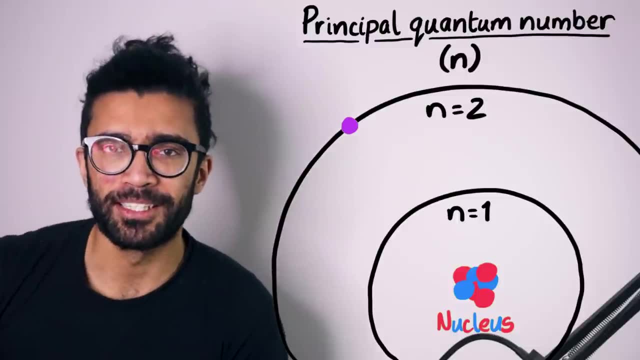 electron is in. if we give the electron a number of n is equal to one, then that tells us that it's in the first shell, and if we assign it n is equal to two, that's because it's in the second shell. the next property that we can discuss: 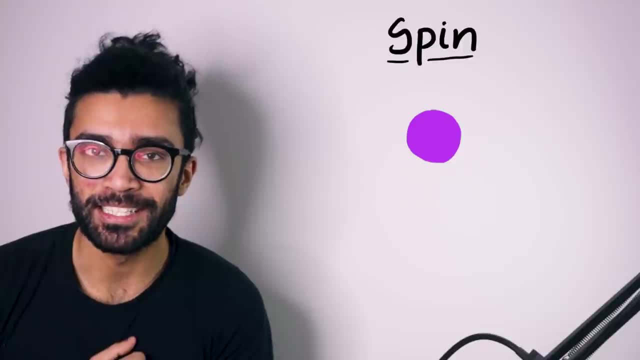 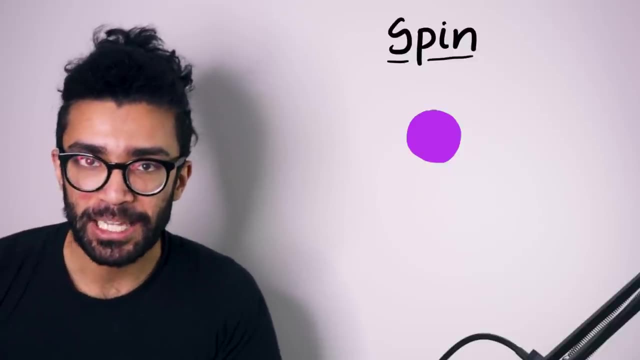 is known as the spin of an electron. you may be familiar with the idea that electrons can be found in one of two different spin states. these are often called spin up and spin down. these can be labeled with the spin quantum number, often called m subscript s, and if the electron is in the spin up state, then 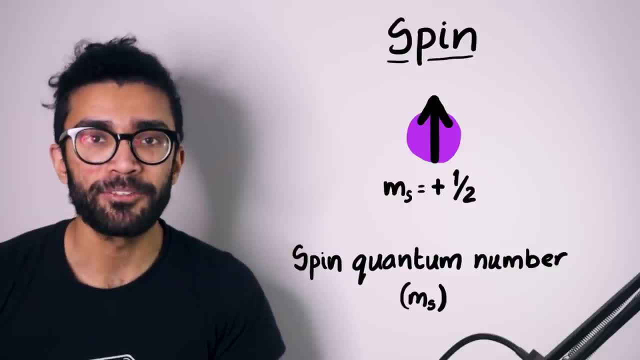 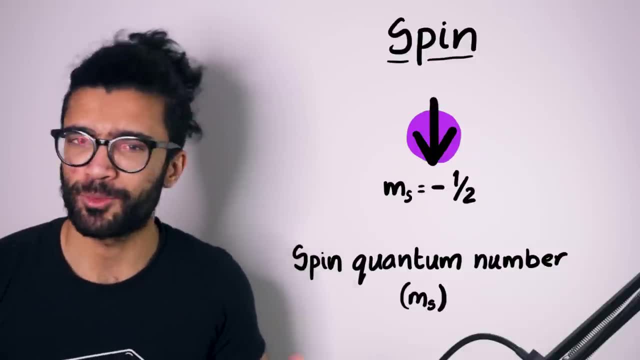 it's given the label, ms is equal to plus one half, and if it's in the spin down state, then it's ms is equal to minus one half. and the reason for using plus half and minus half rather than like plus one or minus one is because electrons have a spin of half. 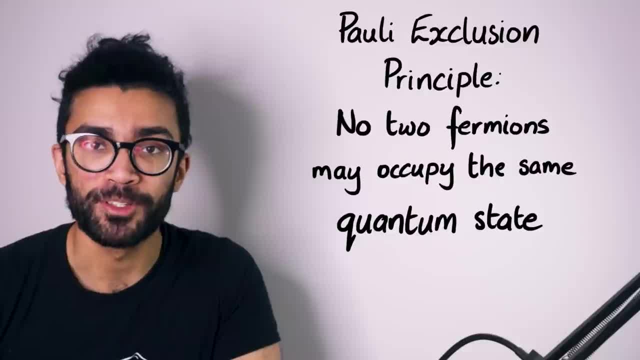 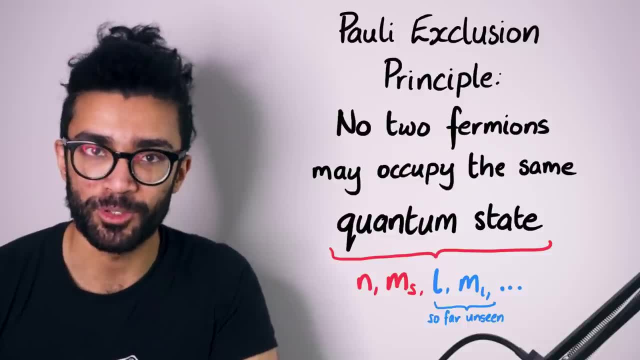 now, the Pauli exclusion principle tells us that no two fermions can be in the exact same quantum state, and the quantum state is described by this set of numbers, of which we've only discussed two so far. what this means is that no two fermions, no two electrons, can have exactly the 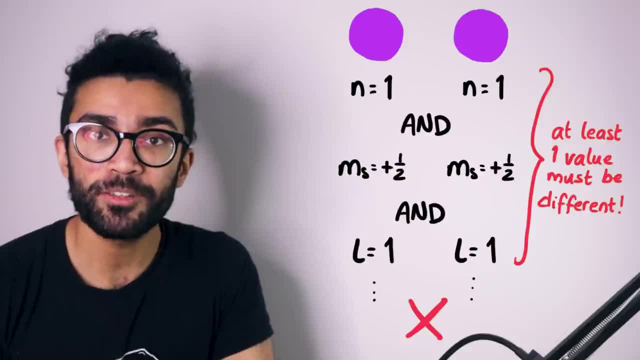 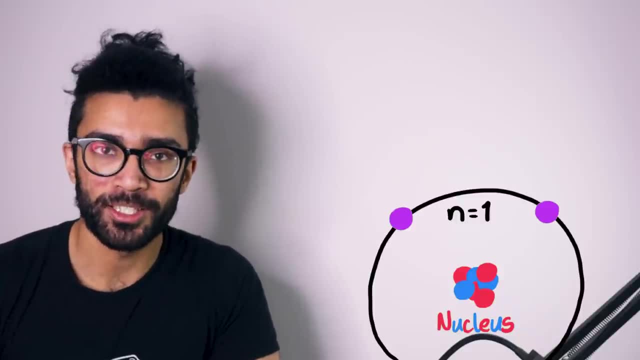 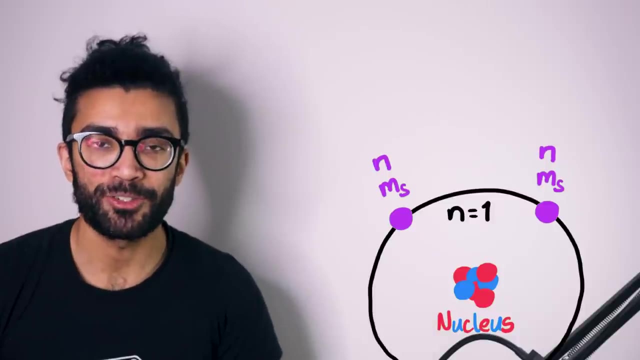 same set of numbers describing them. in other words, at least one of these numbers must be different. now, for the n is equal to one energy level. that's the lowest shell. the only really important numbers are the principal quantum number, n, and the spin quantum number, ms, because in this shell all of the electrons have the principal quantum. 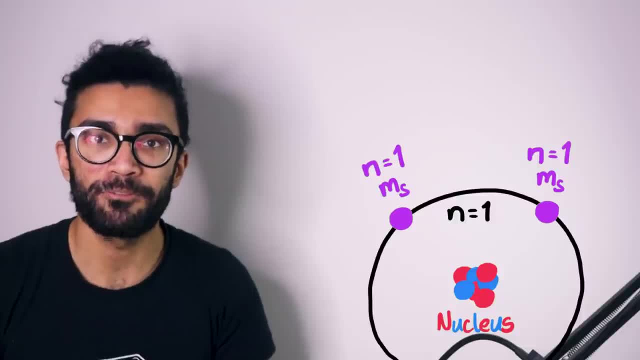 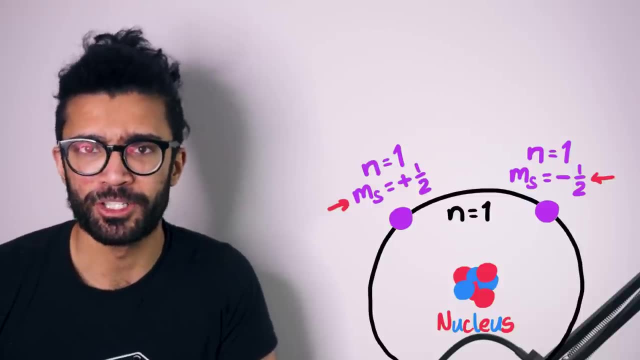 number one because it is the lowest shell. that means that they must have different ms values, and the only two possible ms values are plus half and minus half. therefore the n is equal to. one shell can only hold two electrons. now for higher shells it gets a bit more complicated. we have to consider a few. 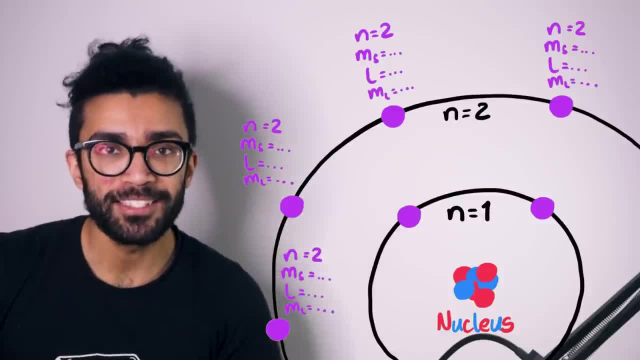 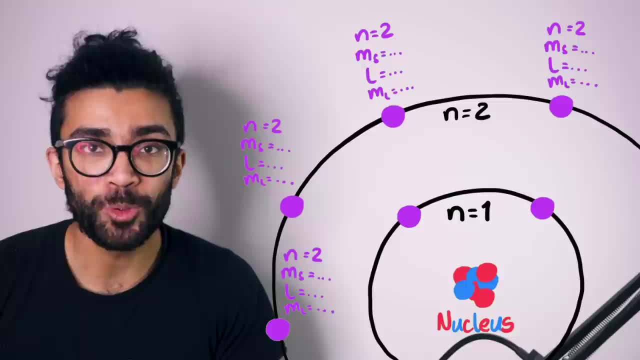 other quantum numbers, which is why there is room for eight different electrons in the second energy level rather than just the two, like we saw in the first energy level. it's worth noting, by the way, that these new quantum numbers can also be assigned to the electrons in the first energy level. 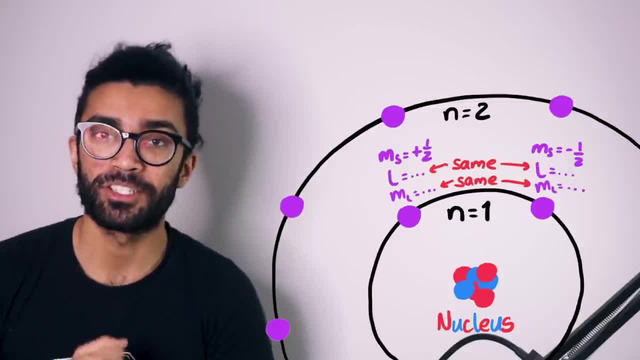 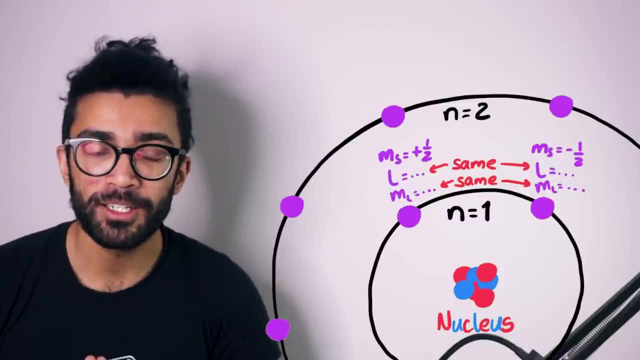 it's just that they happen to be the same for both electrons, and because the condition is that at least one of these numbers must be different, and the only one that can change- for the n is equal to one level- is the spin quantum number. that's why we have room. 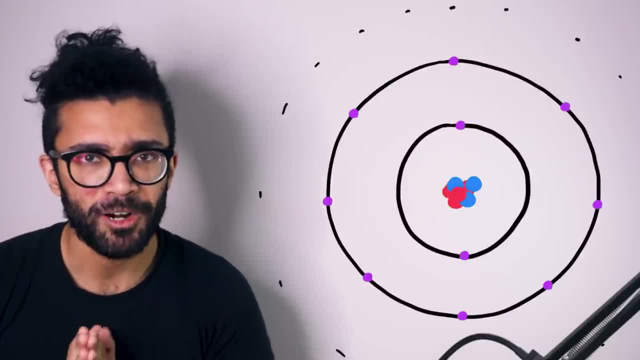 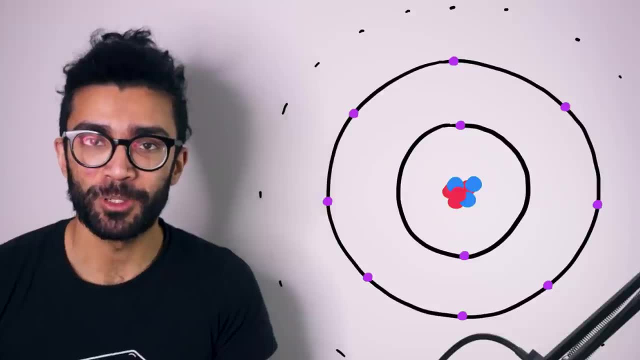 for two of them in there. so this explains why all of the atoms that we see around us have an electronic structure that is divided up into lots of different energy levels. it also explains why each energy level is only allowed to have a certain number of electrons in it, and no more if electrons were bosons instead of. 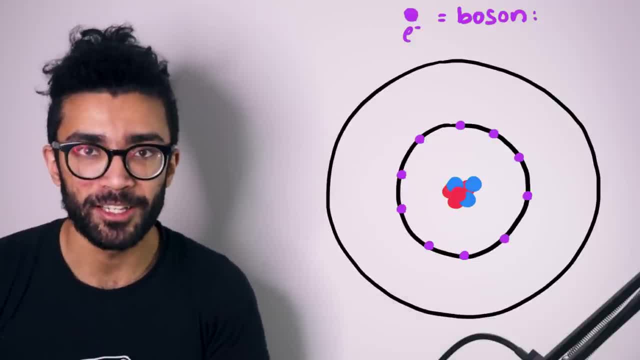 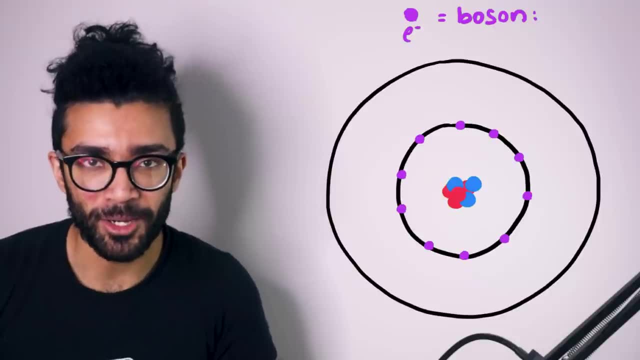 fermions, they would all be allowed to collapse into the lowest energy level, as i've discussed in my bose einstein condensate video, and this would not be good for the atomic structure, or at least the atomic structure as we know it, because chemistry as we know it would 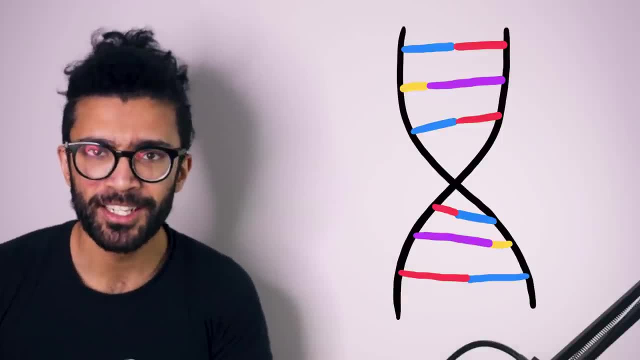 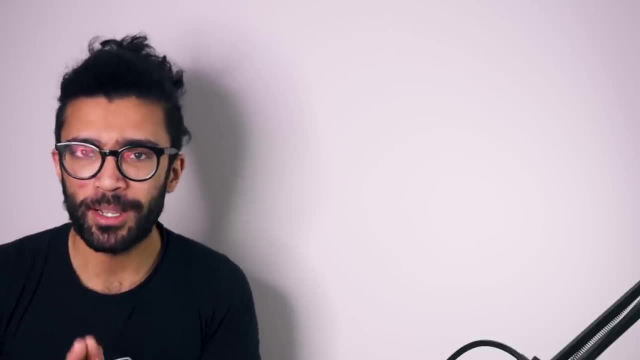 not exist, and therefore biology as we know it would not exist, and perhaps life as we know it would not exist, and i find this quite profound, to be honest, in order for the universe around us to be the way it is, assuming our understanding of quantum mechanics is at least relatively correct, 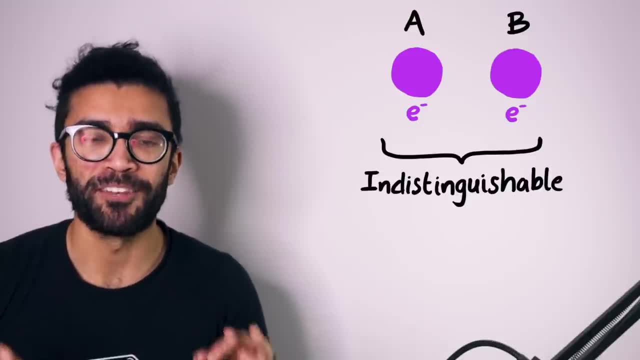 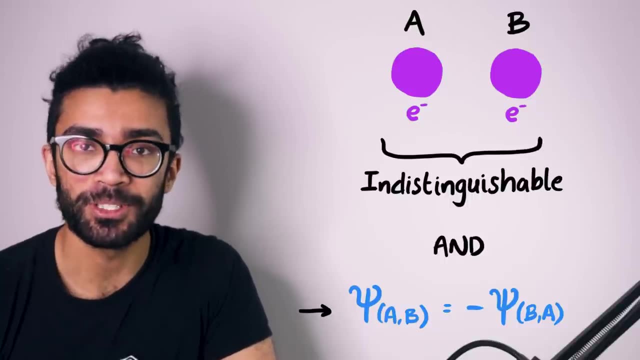 electrons have to be indistinguishable from each other, and very specifically the fermionic kind of indistinguishable, not the bosonic kind. and not only that, but this simple mathematical condition is enough to explain the behavior of electrons in atoms. how cool is that. and with all of that, 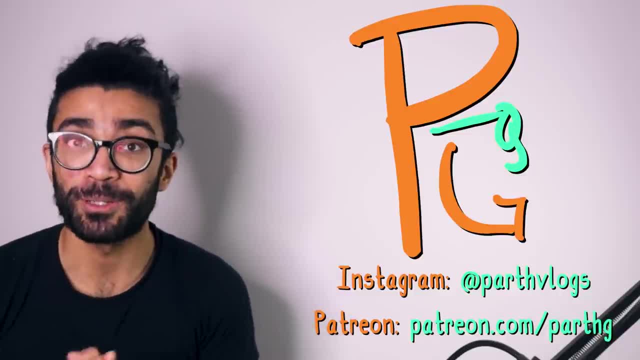 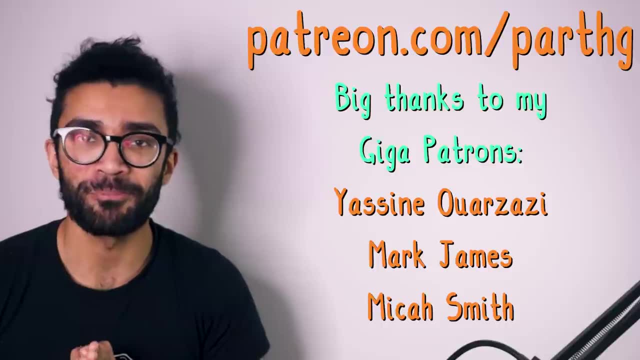 being said, i'm going to finish up here. thank you so much for watching. if you enjoyed the video, please do hit the thumbs up button and subscribe for more fun physics content. hit that bell button if you'd like to be notified when i upload, and please do check out my patreon page. 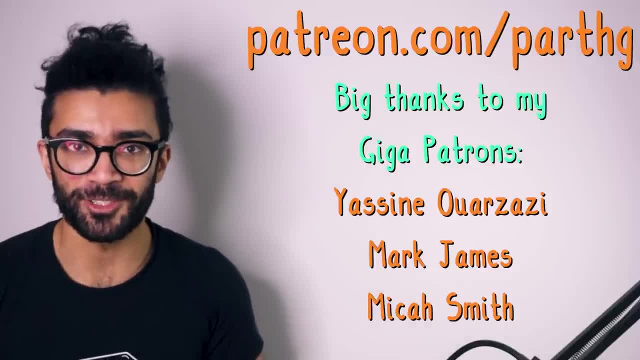 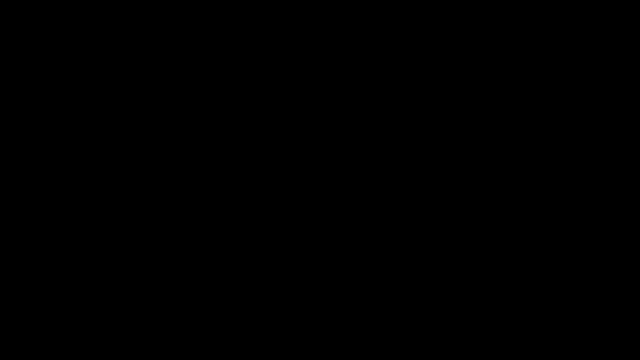 if you'd like to support me on there. thank you so much for watching and i'll see you very soon. you.